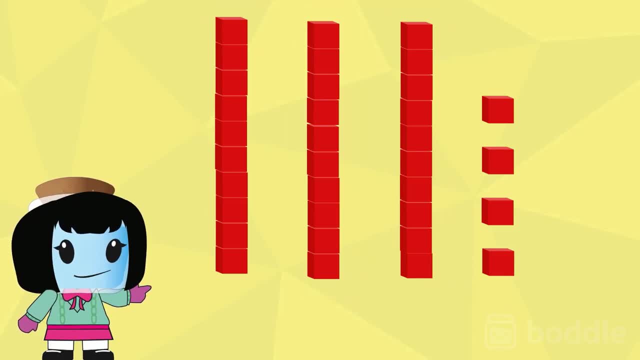 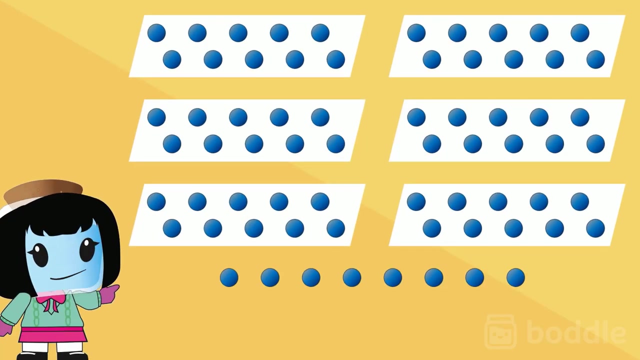 have ten blocks each. Well, there are four blocks that are not stacked into blocks of ten. We can say that the stacks are three tens and the separate blocks are four ones, which means we have 34 blocks in total. next, let's count the number of tens and ones from the dots below can. 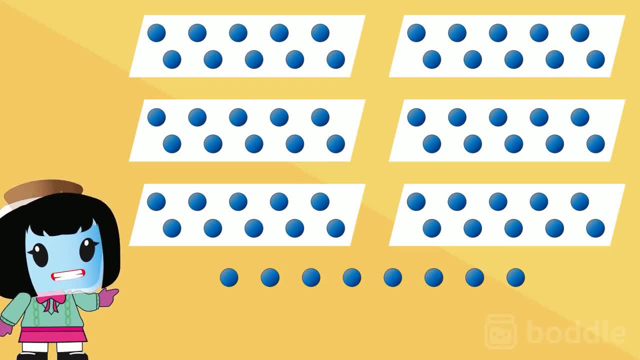 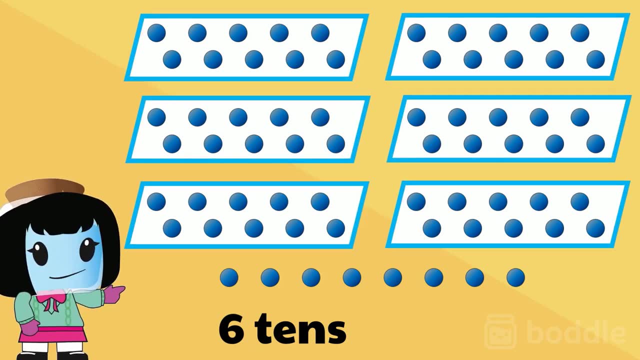 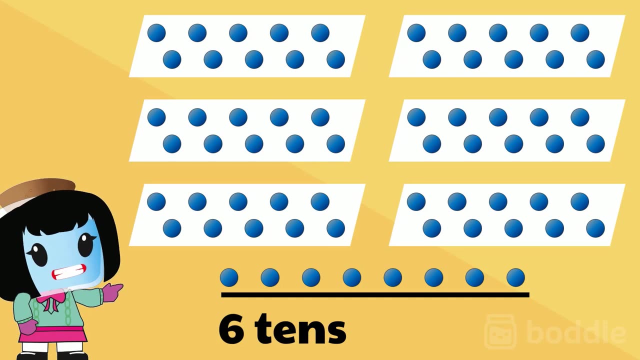 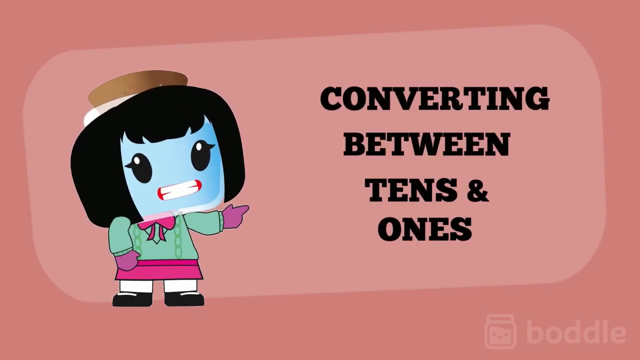 you guess how many tens we have here. that's right, we have six tens because there are six boxes that have ten dots each. notice that there are eight dots that are not boxed into groups of ten, so we have eight ones. in total, we have sixty eight dots. now let's try converting between tens and ones. match the tens to. 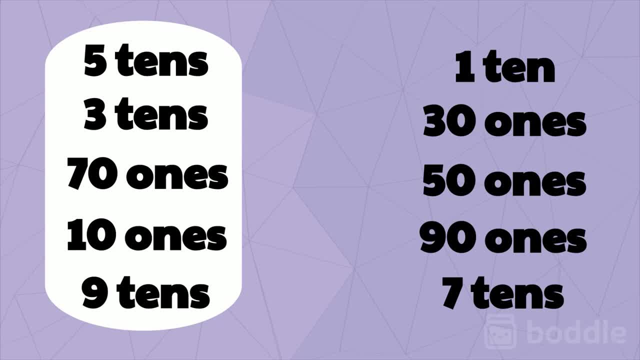 the ones or the ones to the tens. five tens is equal to 50 ones. three tens is equal to 30 ones. 70 ones is equal to seven. ones is equal to 50 ones. three tens is equal to 30 ones. 70 ones is equal to 7. 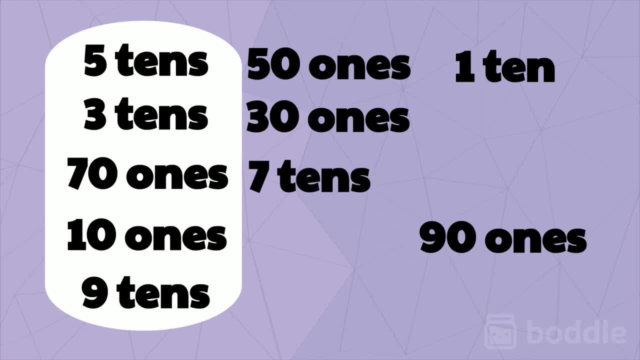 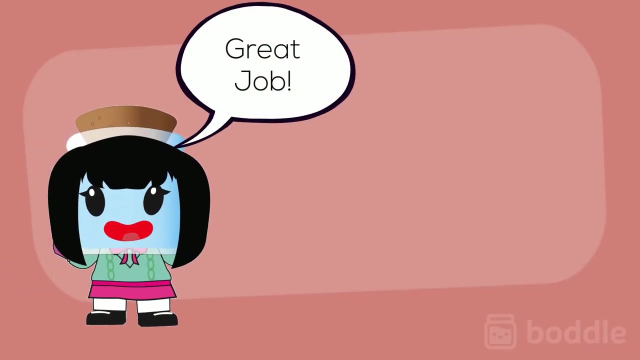 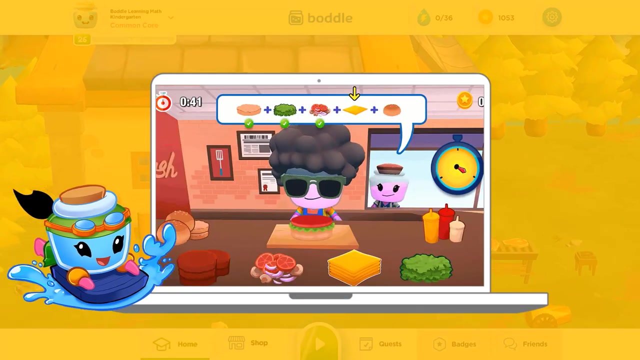 ones is equal to 7 10s. 10 ones is equal to 1- 10. 9 tens is equal to 90 ones. great job working with place value. see you again soon. are you looking for more fun ways to learn math? check out, bottle learning and access thousands of math. 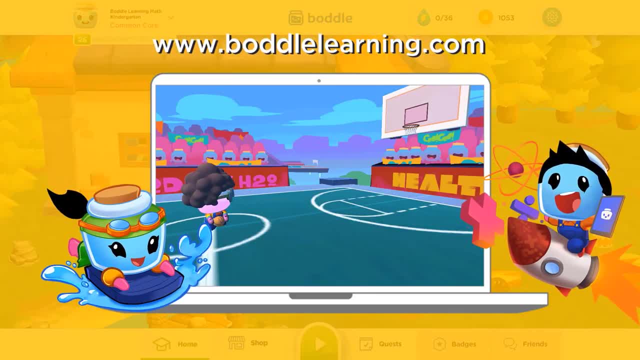 skills all through a fun 3d game. just visit bottle learning calm and sign up today.